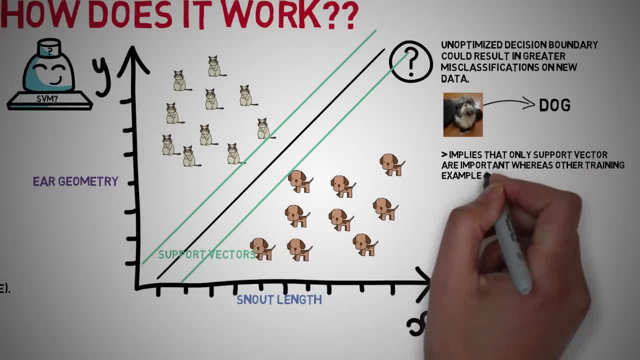 support vectors are important, whereas training examples are ignorable. An example of this is so that if we have, in our case of a dog that looks like a cat, or a cat that is groomed like a dog, we want our classifier to look at the extremes and set our margins based. 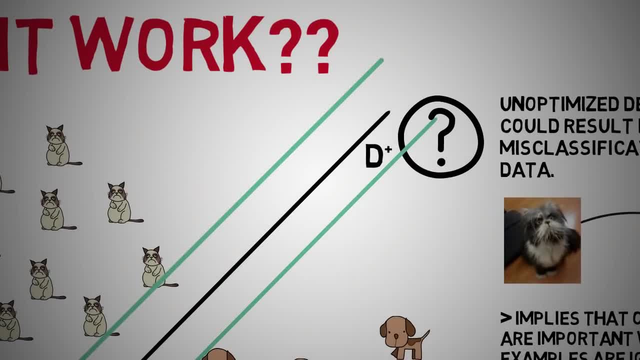 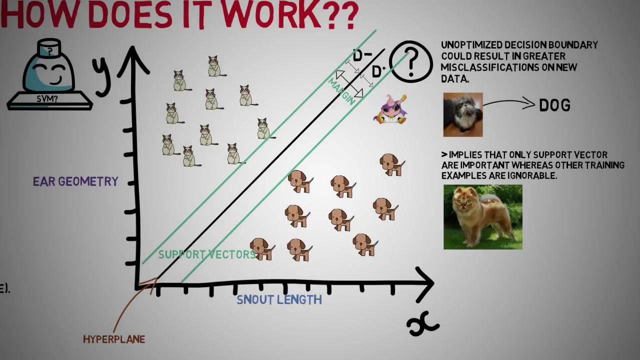 on these support vectors. The line or decision boundary that segregates the two classes is commonly referred to as a hyperplane, because SVMs can be used in multi-dimensional data sets and the data points are referred to as vectors as they have coordinates within this space of data. 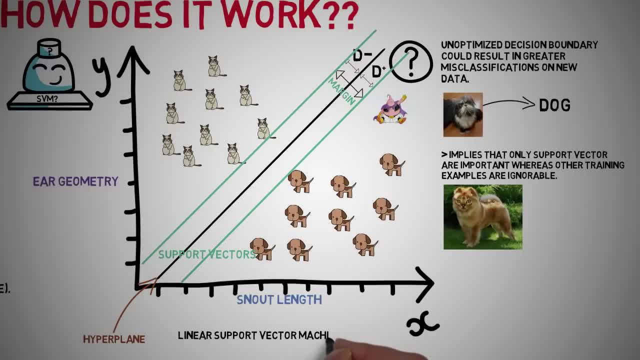 So what we discuss so far is also known as linear support vector machines or LSVM, because the classes are linearly separable. But what happens if we have a data set that is not linearly separable? So say, we are presented with data that looks like this, where it looks: 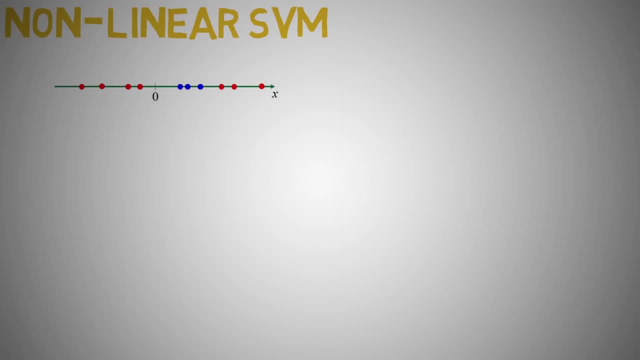 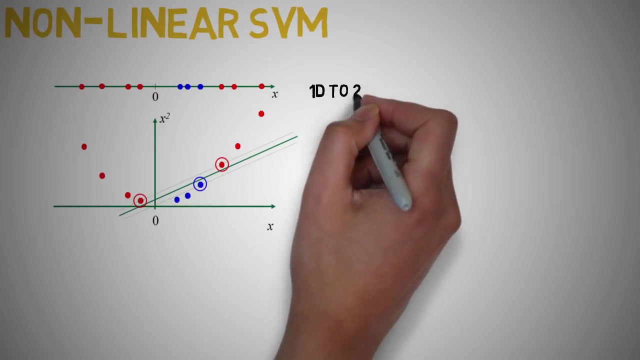 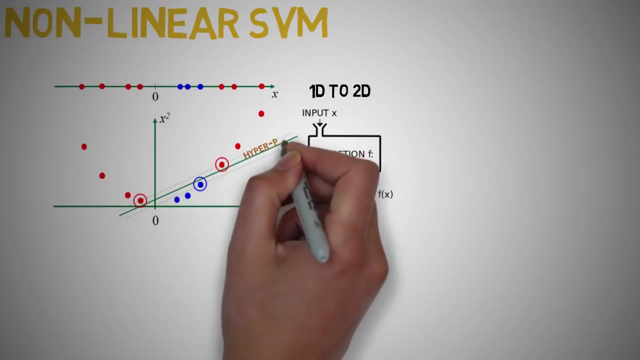 almost impossible to use a single line to separate the two classes. We can use a function to transform our data into higher dimensional space. So you can see, over here we go from two dimensional space. We can apply a simple polynomial function to get a parabola and. 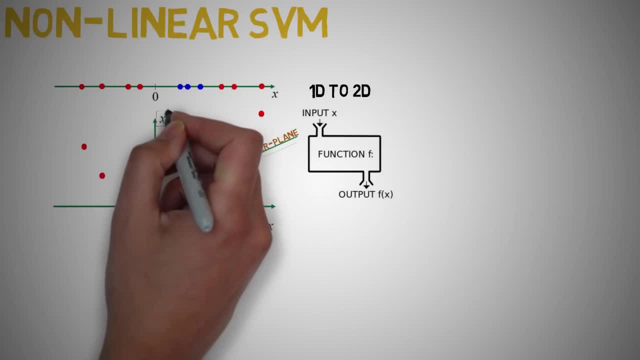 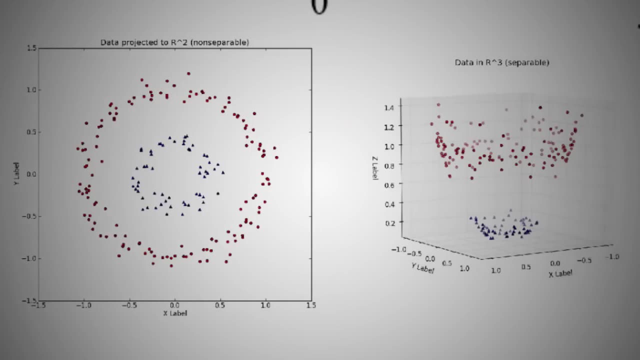 now you can easily see how we can draw our hyperplane. We can do the same for this data set, where it's easy to draw the hyperplane or line. but for a machine we'd use a function to transform our data from two dimensional to three dimensional feature space. 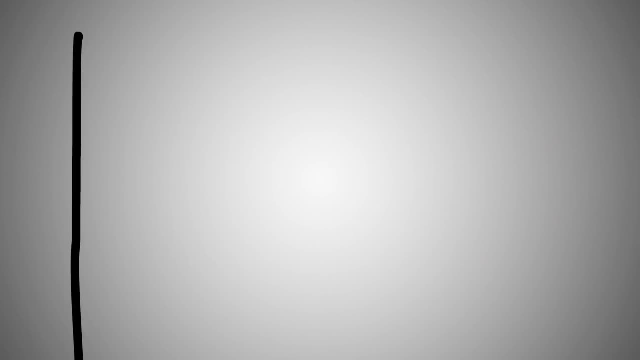 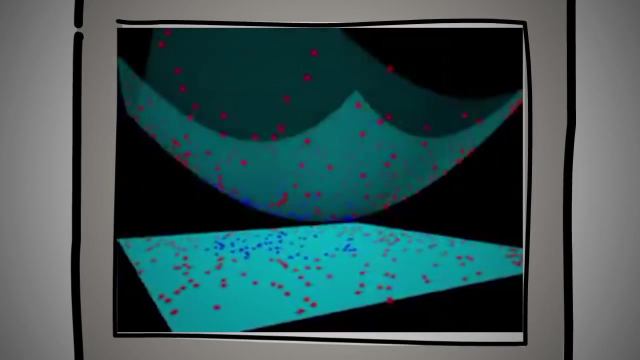 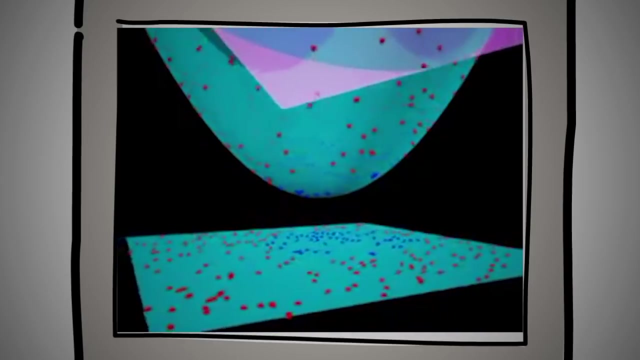 Now, the only problem with transformation into higher dimensional feature space is that it's computationally expensive. We can use a kernel trick to reduce the computational costs. So let's take a look at a function that takes as its inputs vectors in the original space and returns the dot product of the vectors in the feature space is called a kernel function. 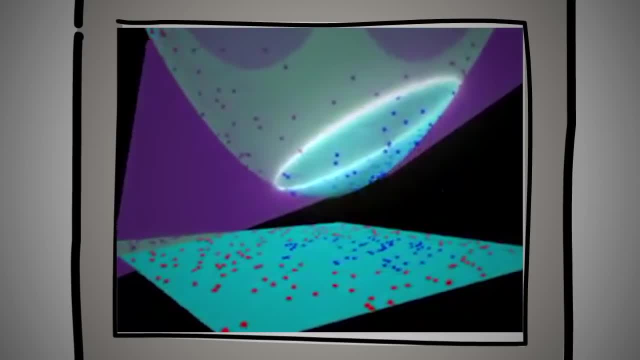 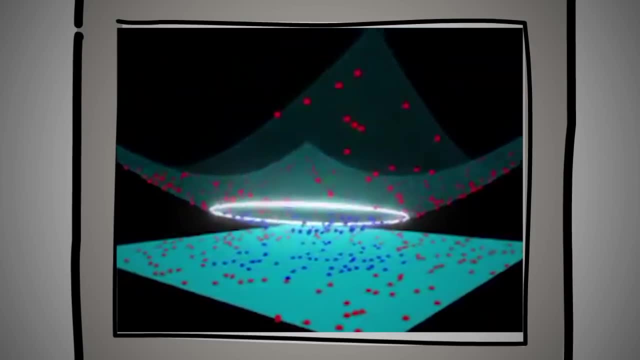 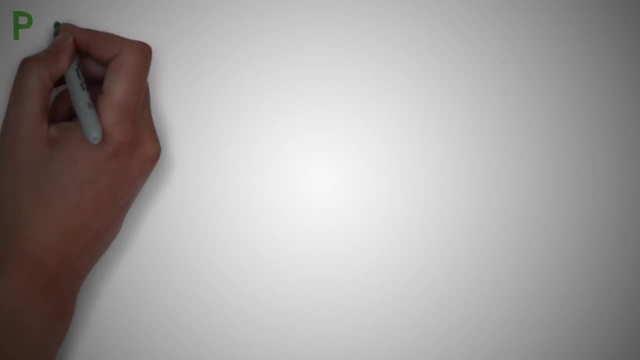 also referred to as kernel trick. Using a kernel function, we can apply the dot product between two vectors so that every point is mapped into a higher dimensional space via some transformation. So essentially we use it to transform a non-linear space into a linear space. 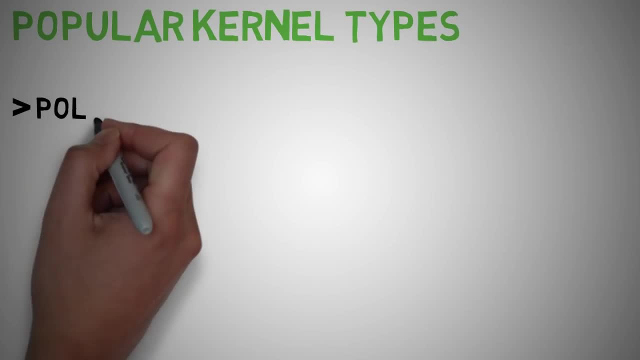 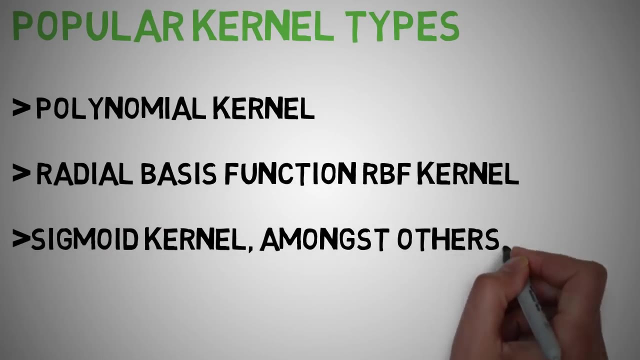 If we look at some popular kernel functions, we can see that the kernel function is called kernel types. Here are some popular kernel types that you can use to transform our data into higher dimensional feature space. There are polynomial kernel, radial basis function, sigmoid kernel, amongst others. Unfortunately, choosing the correct kernel 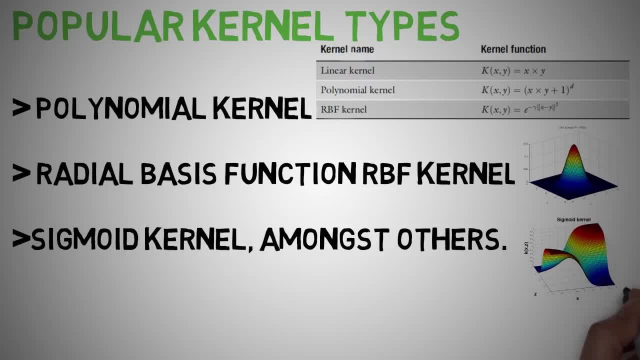 is a non-trivial task and may depend on specific tasks at hand. No matter which kernel you choose, you need to tune the kernel parameters to get good performance from your classifier. A popular parameter tuning technique is called the R-BF kernel. This is a very popular method. 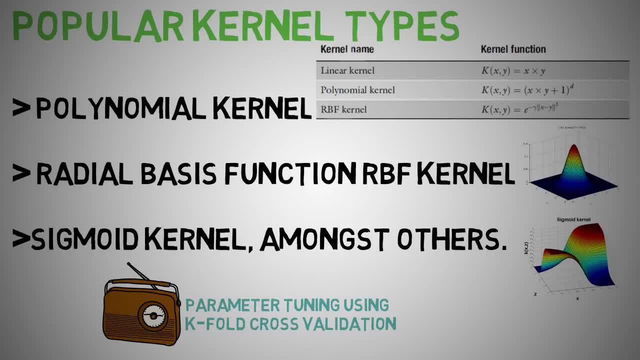 of tuning the kernel parameters to get good performance from your classifier. A popular parameter tuning technique is called the R-BF kernel. This is a very popular parameter tuning technique. A popular parameter tuning technique includes k-fold cross validations. We'll deal with some of these parameters in our Python labs. 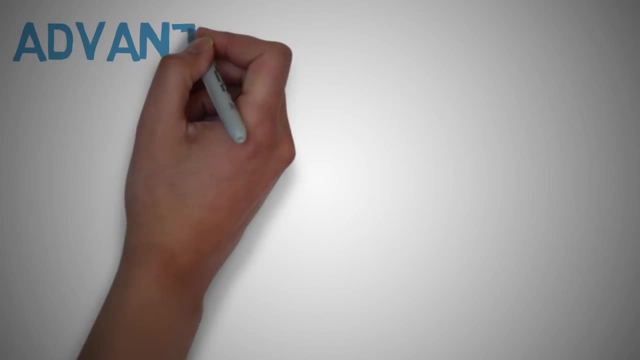 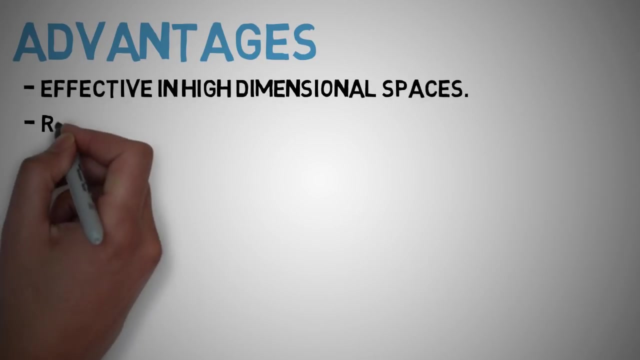 So the advantages of support vector machines are that they are effective in high dimensional spaces. They are still effective in cases where the number of dimensions is greater than the number of samples. They use a subset of training points in the decision function or support vectors, so it is also memory efficient. 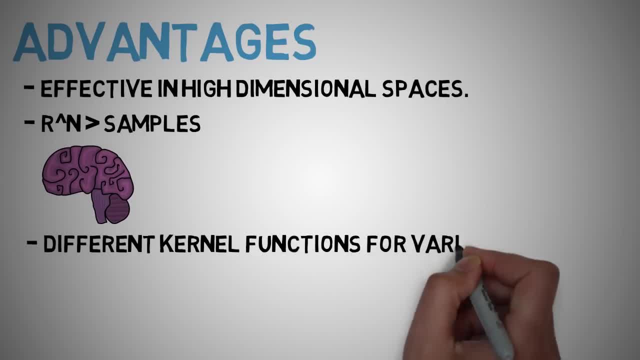 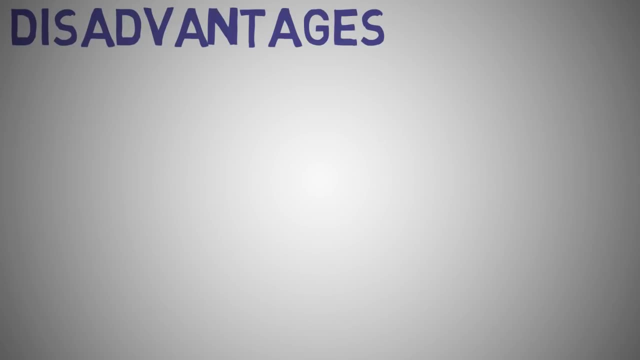 Support vectors are versatile, So different kernels can be specified for the decision function. common kernels are provided, but it's also possible to specify custom kernels. we can add kernel functions together to achieve even more complex hyperplanes. the disadvantages, however, of support vector machines include, if the 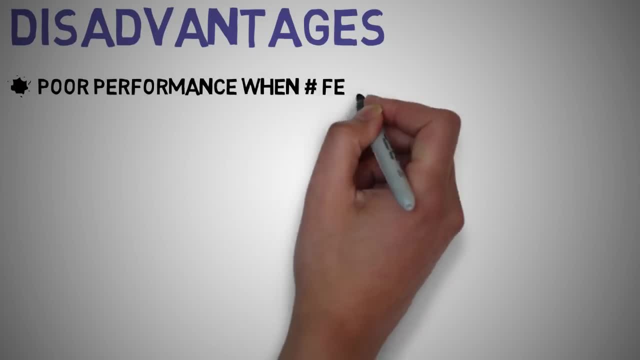 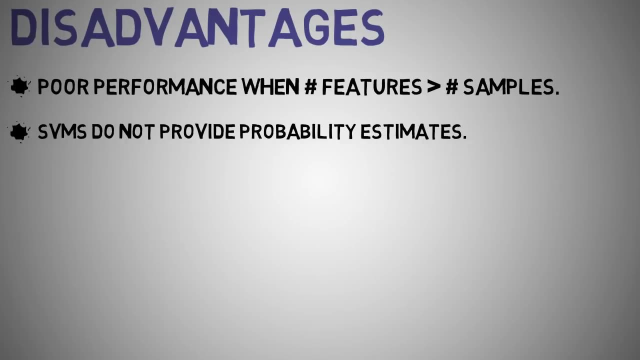 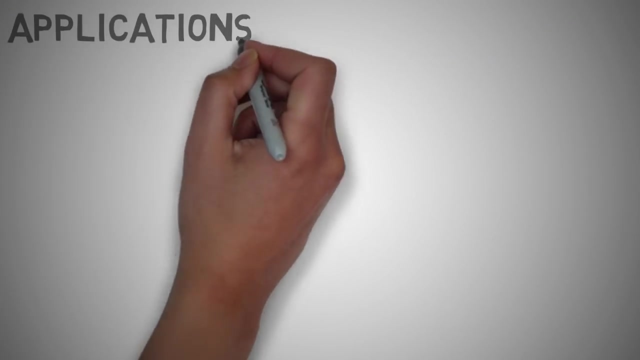 number of features is greater than the number of samples, the method is likely to give poor performance. support vector machines do not directly provide probability estimates. these are calculated using an expensive five-fold cross-validation. if you take a look at the applications of support vector machines, the support vector machine algorithm has numerous applications and 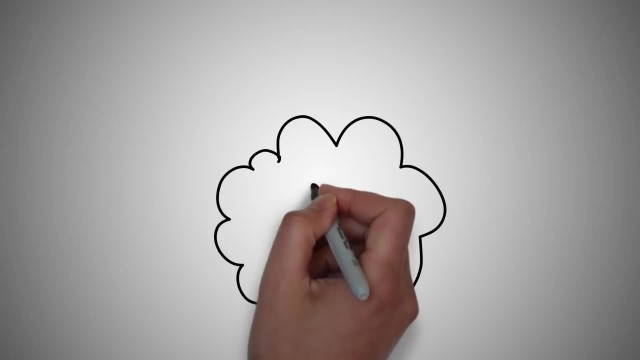 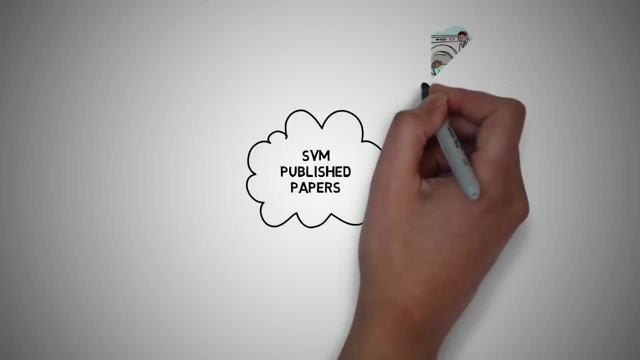 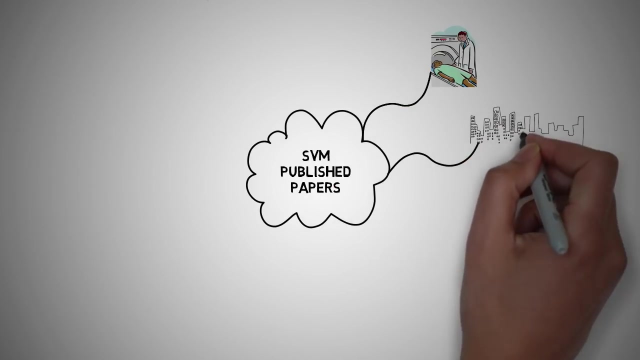 can be a quite popular alternative to artificial neural networks or ANNs. here are some applications from published journal papers so we can use support vector machines in medical imaging. there's one application for SVM based regression models to study the air quality in urban areas in the city of 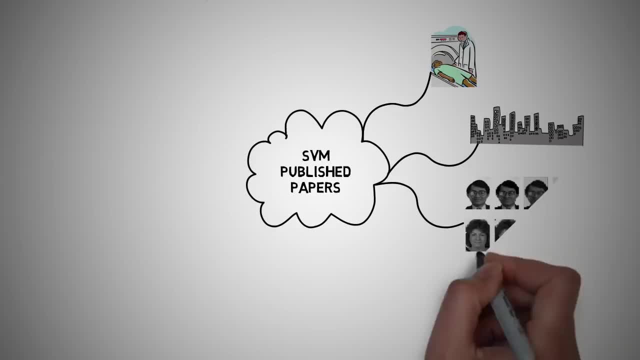 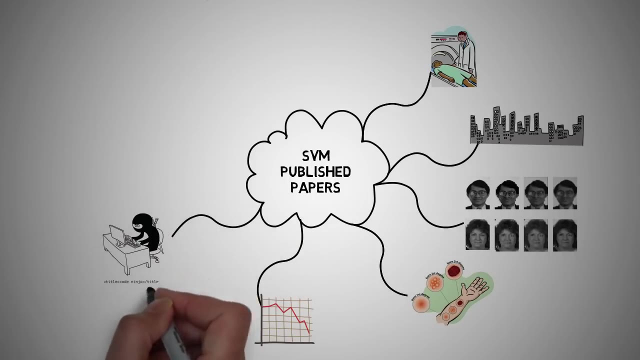 Oviedo in Spain. support vector machines is also used for image interpolation as well as medical classification tasks. in the financial industry, support vectors are used for time series predictions as well as financial analysis. there's one paper on the application of neural networks mixed with support vector machines in